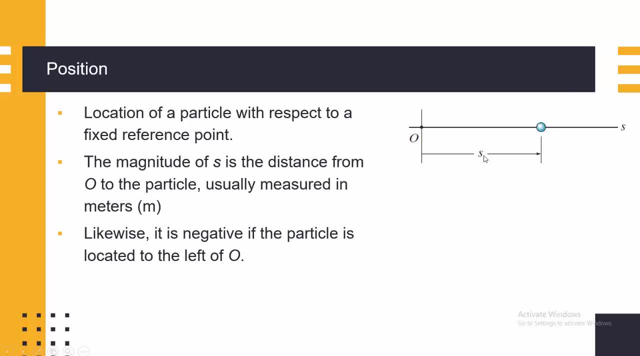 The particle is located at a distance of s from the origin. Generally, the position is measured from the origin. In most of the cases, the origin will be 0, 0.. So here s is the position of the particle. Here the s is positive. That is why the particle is on the right side. 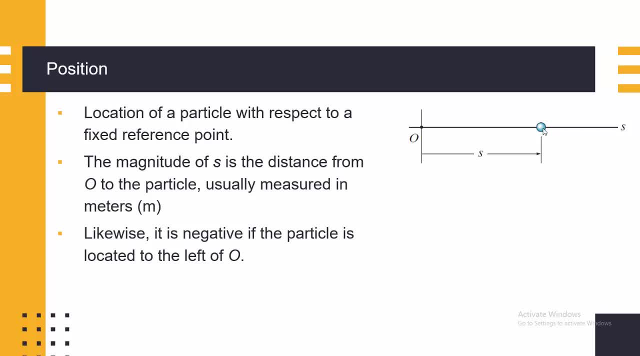 If it is negative, then the particle will be at the left side. The example for position is: the car is placed at a distance of s from the electric pole. So here the s is the position of the car and position means it is the distance. 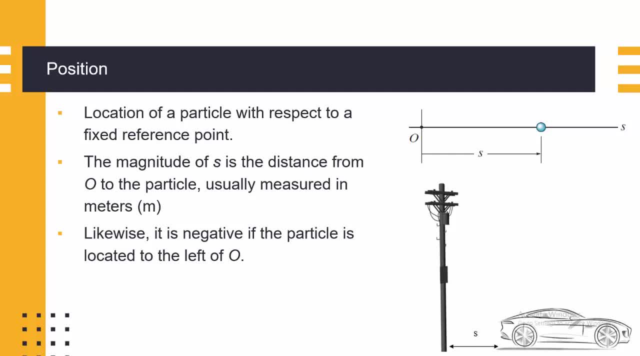 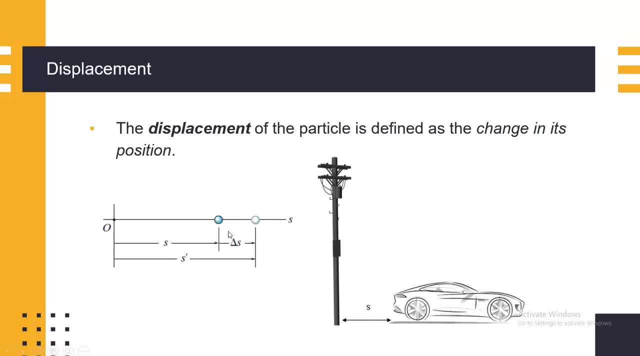 So the distance is generally measured in meter. So also the position is also measured in meter. Then the displacement, So here the particle moves from the position s to s dash. So the difference between s, dash and s is delta s. So that is the change in position. 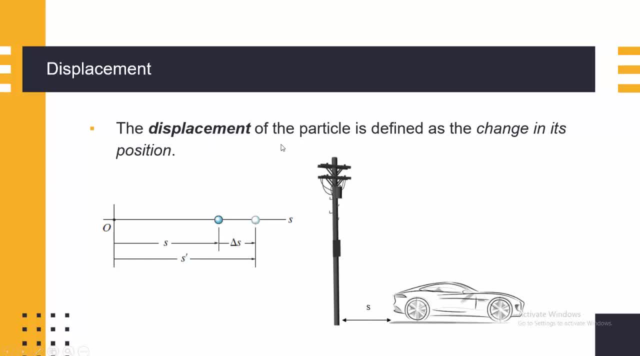 So this change in position is called as displacement. So displacement of the particle is defined as the change in its position. In this example the car is located at the distance. If the car is moved to s dash, then the difference between s dash and s is the displacement. 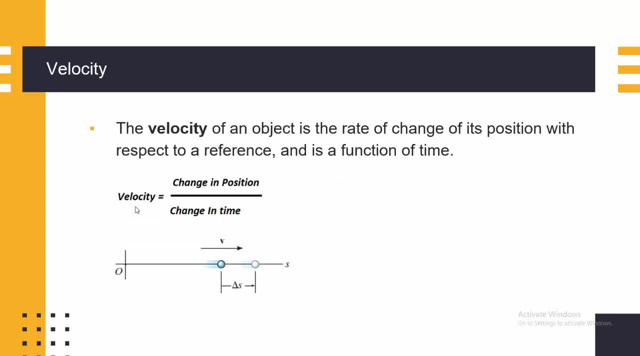 So the unit for displacement is also meter. Next is velocity. The velocity of an object is the rate of change of its position with respect to time. Here the object is moving from its first position to the final position. So to move this distance. 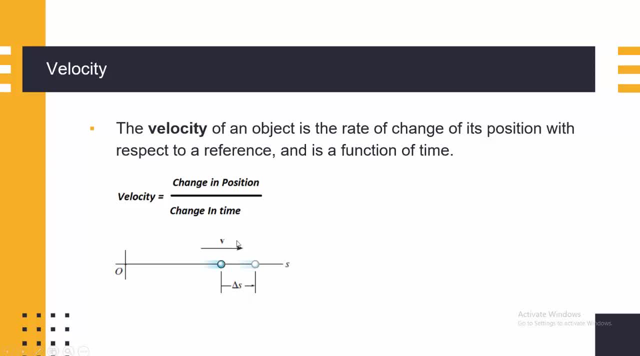 Delta s in a period of time it has some velocity. If the velocity is high, then the particle will move in a less time. If the velocity is low, then the particle will move in a very long time. So here, car is moving with some velocity from s to s dash. 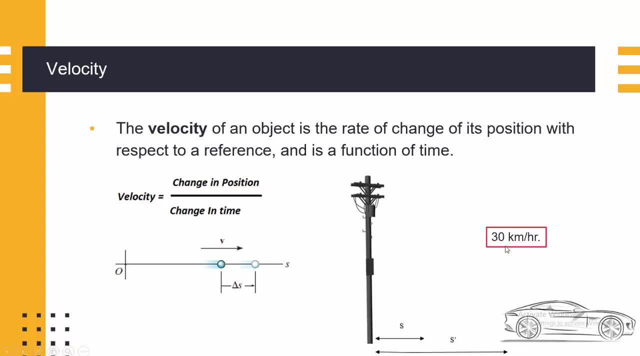 So mostly in automobiles we will specify the speed by kilometer per hour. For example, consider the car is moving at speed, The speed of 30 kilometer per hour. The meaning for 30 kilometer per hour is if the car is operated at a constant velocity, then this will cover a distance of 30 kilometer in one hour. 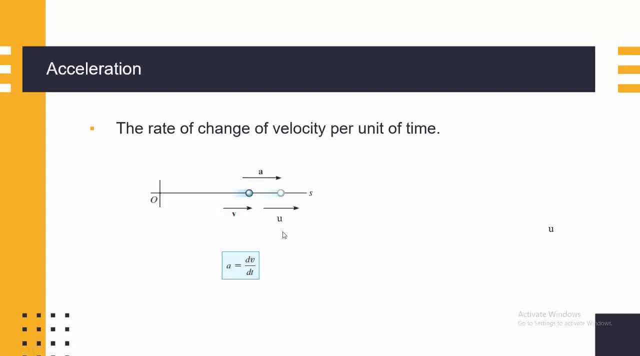 So that is the meaning for 30 kilometer per hour. Next is acceleration. So acceleration is the rate of change of velocity with respect to time. So at the initial position, the particle is having a velocity of v And at the final position, the particle is having a velocity of u. 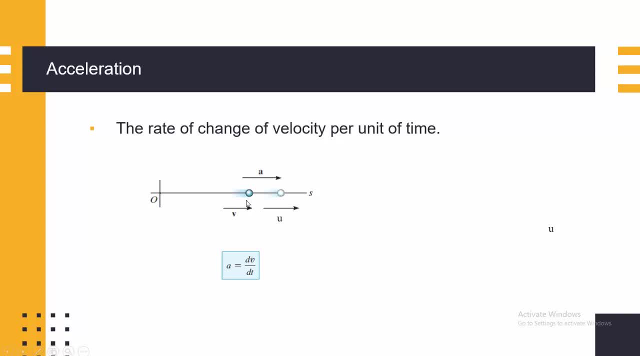 In between these two positions, its velocity is changed, So we can consider that its velocity increases, So that rate of change of velocity is called as acceleration. So if the acceleration is high, then the change in velocity, or increase in velocity, will be high. If the acceleration is low, then the increase in velocity will be slow. 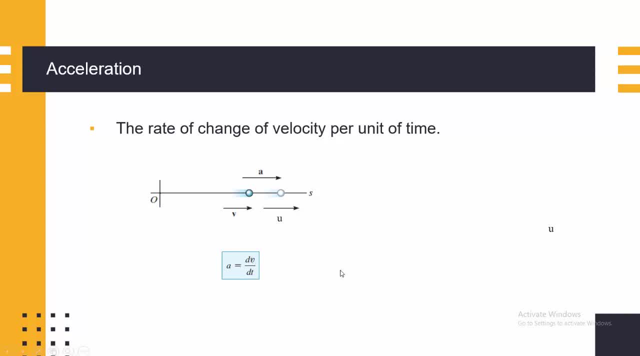 So a is equal to dv by dt In automobiles. if we apply throttle, then we are increasing the velocity. For example, we are increasing the velocity from 10 kilometer per hour to 40 kilometer per hour. In the same time, if you apply brake, then we are reducing the speed from 40 kilometer per hour to 0 kilometer per hour. 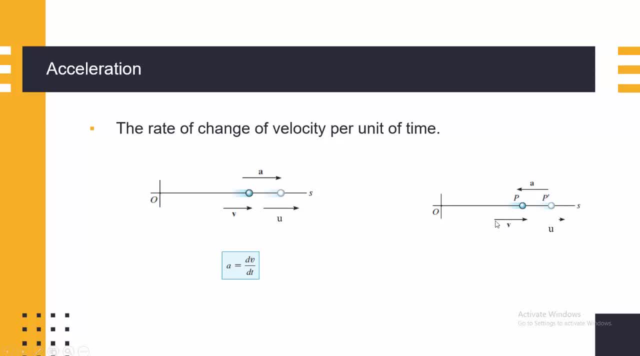 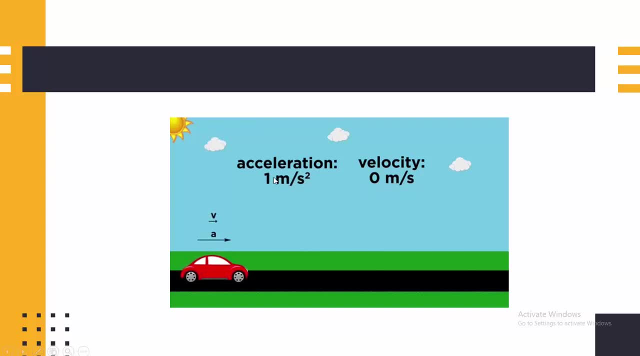 So that is the difference between acceleration and retardation. So with this example you can see, You will get a clear idea about acceleration and velocity. So initially a 1 meter per second square acceleration is applied, So the velocity is increasing from 0 to 1.. 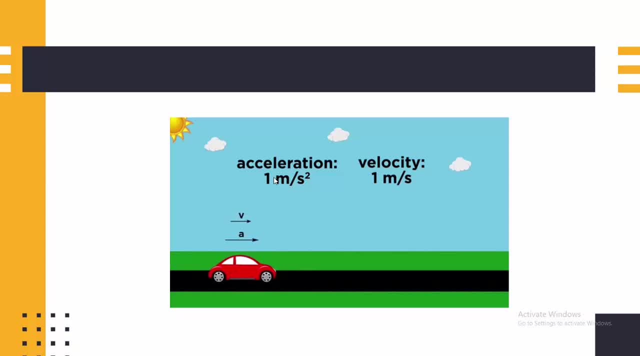 I am continuously applying the acceleration, So the velocity is increased to 2.. Further I am applying the acceleration, The velocity is increased to 3.. Further it is increased to 4.. Further it is increased to 5.. And now I am applying the brake.